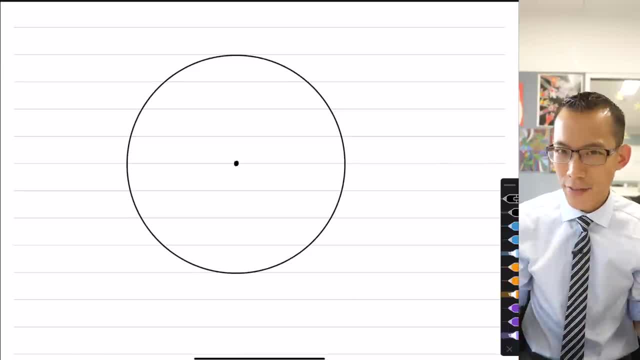 is the first time I encountered it, So, without giving more preamble, let me tell you about the particular property that I'm interested in. It's about what we call the angle in a semicircle. So if you take any circle and you draw any diameter so you can see, I've already marked the center. 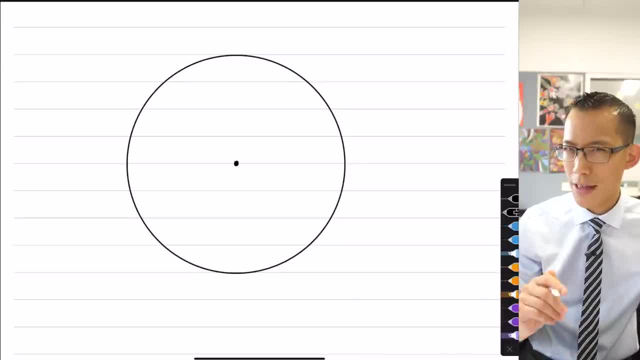 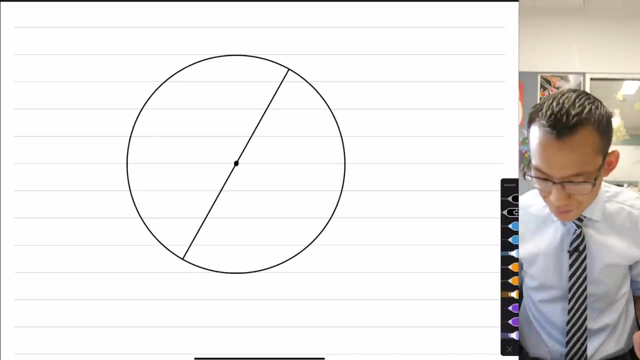 of this circle. so if I draw a chord that passes through that center, it'll be a diameter. So if I say, for example, place a, let's get a straight line here, place a chord right through the center, like so okay, fantastic, so this is a diameter. now, if I then take this diameter and use its ends, like 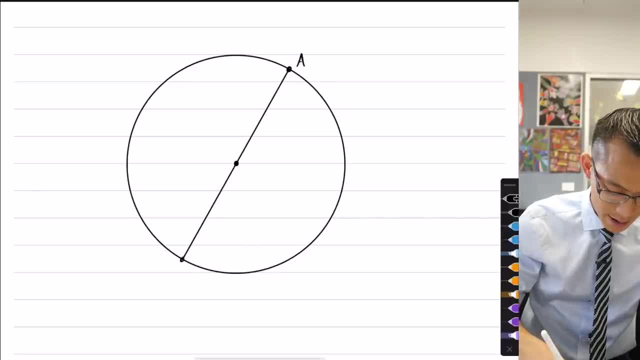 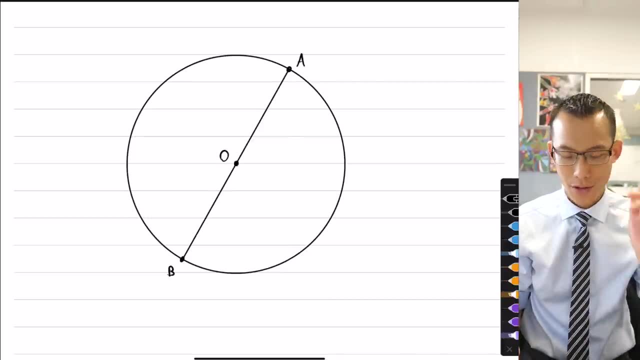 if I call this diameter, diameter a, b, and then I've got the the center of the circle o there, okay, if I pick any other point on the circle anywhere on the circumference, I should say, say, for instance, a point like, say here, then if I join up an angle from a to that point, 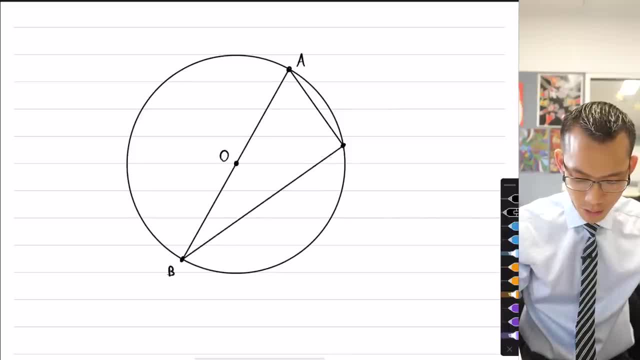 and then go from b to that point and let's call this new point p, one of the things you'll notice. and if you've drawn a circle yourself at home and you've picked some arbitrary diameter a, b and some arbitrary point p- I could put this anywhere that I liked- you would actually show. 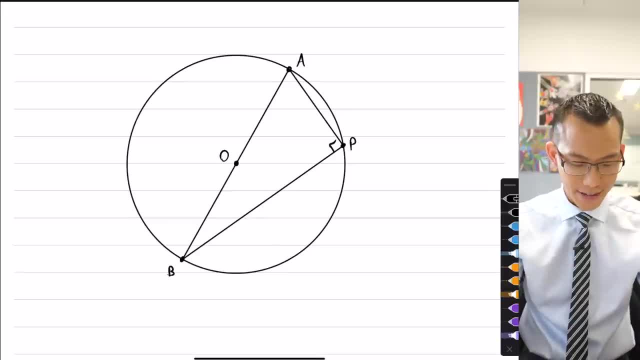 that you always get a right angle and, in fact, a kind of nice, neat illustration for this. let me see if I can actually do it all in one go If I delete my constructions in the manner that I want them to be. I'll just go to the right here and I'll just go to the left here. 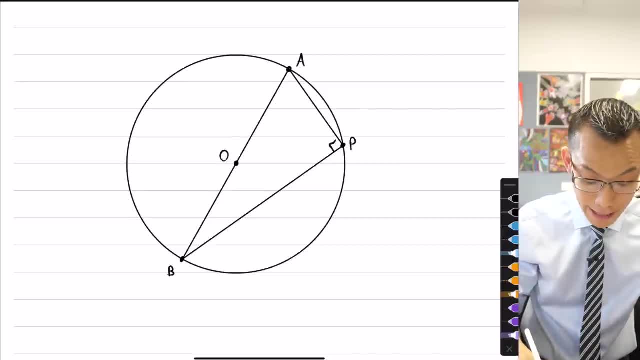 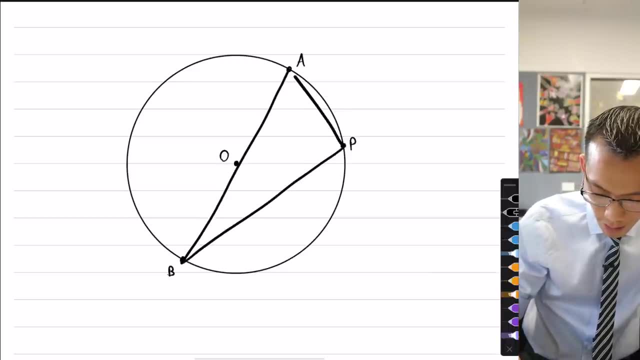 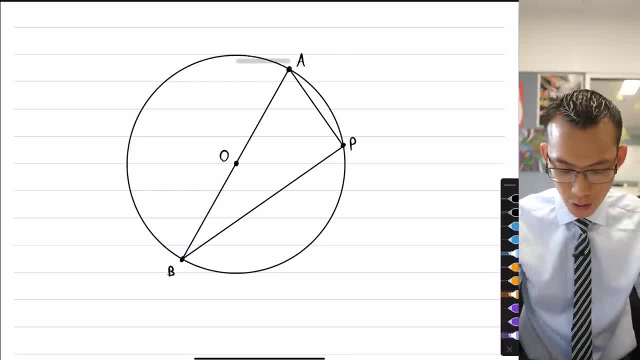 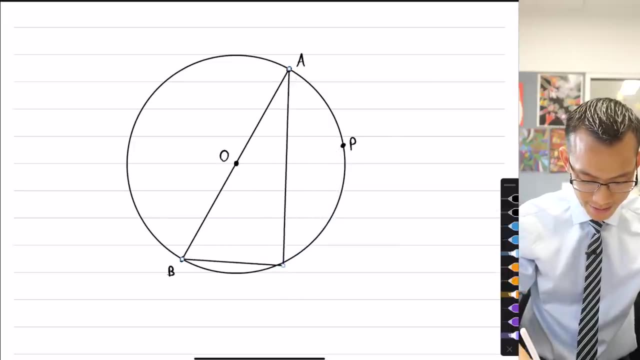 get those spots there. Okay, what I've got now is this ABP triangle and if I just leave A and B fixed but move P around, you can see what I've got here. so long as I move P somewhere along the circumference of the circle and stay on there, can you see wherever you go. you're going to get that. 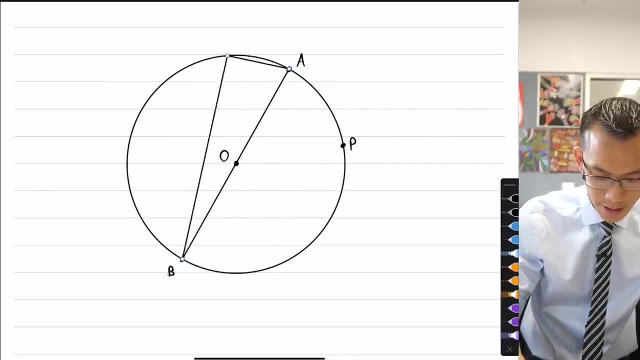 right angle, I can move it even over to the other side. I mean, the symmetry of the circle probably tells you you're always going to get something like that right. So this sort of geometric feature that we notice here- because it is true wherever P. 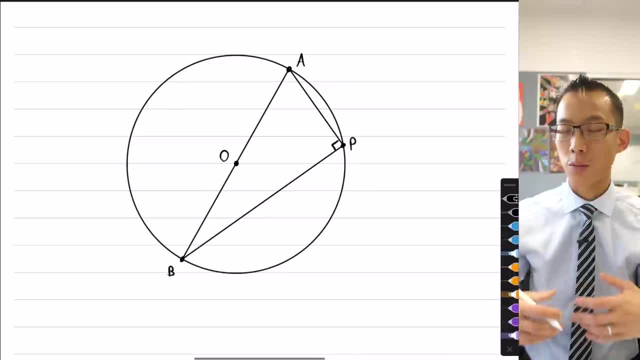 is on the circumference. one of the ways that we can phrase this is that the angle in a semicircle- because AB, the diameter, creates well, creates Two semicircles, but the angle in the semicircle, in this case, APB, it's always going to be. 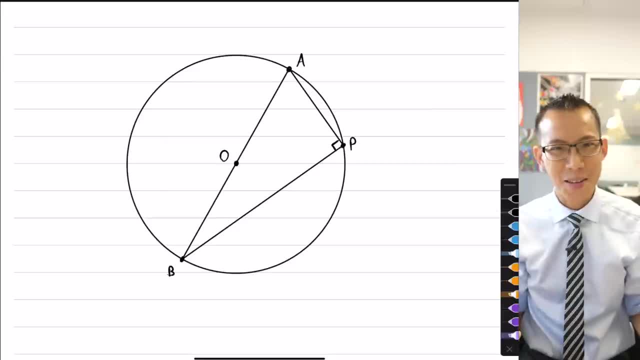 90 degrees. it's always going to be a right angle. Now, this is kind of cute, it's kind of lovely. I think it's really nice because of its simplicity and also it's slightly surprising. but another feature that's really nice about it is it's. 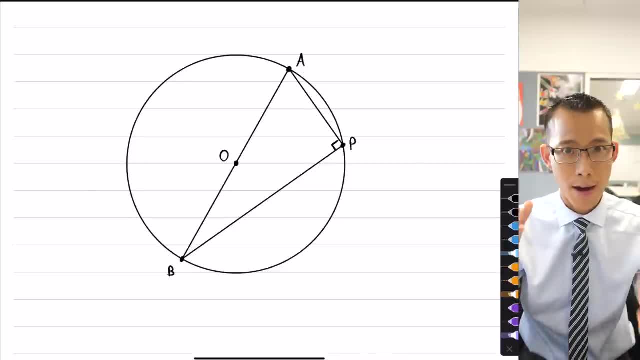 very easy to prove and when I have taught this many times in the past, it's always essential not just to give a property but to say, well, how do I know that that property actually is true? It kind of looks like it and you can draw as many circles and diameters and angles in. 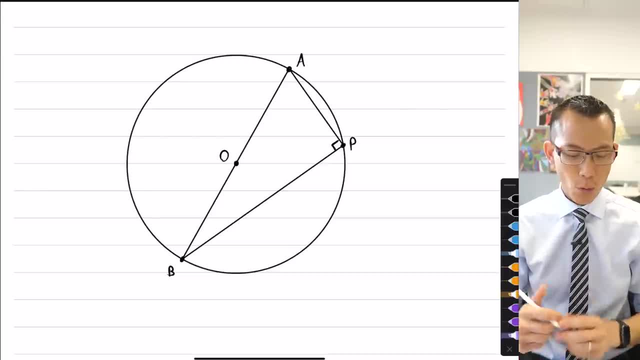 the semicircle that you like, and you'll verify this. but one of the things that sets apart mathematics is that giving examples, even lots and lots, millions of examples, is not sufficient to constitute a mathematical proof. What we look for is a deductive argument. 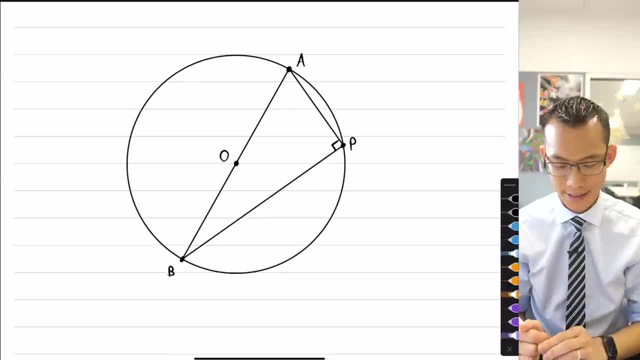 We want to see the logic that proves to us why it is the case. Now, when I've taught this in the past, I have pretty much always done a very, very simple version of the proof that I'm about to show you now, and it's pretty straightforward. 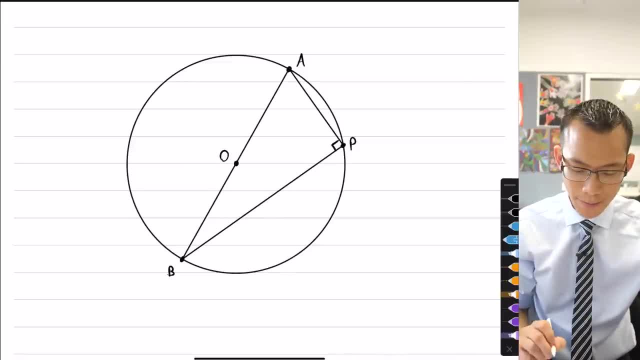 and simple and brief, which is why I've used it so frequently and the way to prove that this angle here A, P, B- is always going to be right angled- just relies on a few basic features of a circle. So let's just suppose we rewind a little bit. 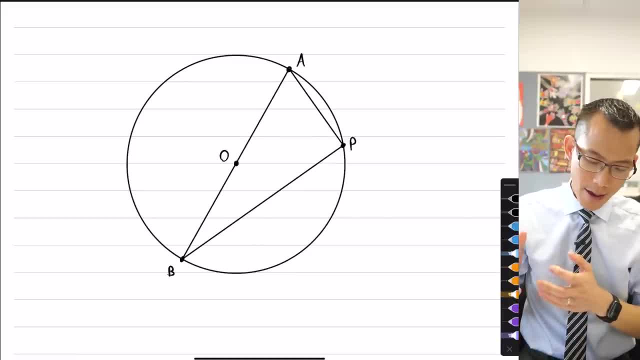 We've created the diameter A, B and we've chosen a point P, and we want to know what is that angle there Like? what is this equal to? If I didn't already know that it was 90 degrees, how could I evaluate it? 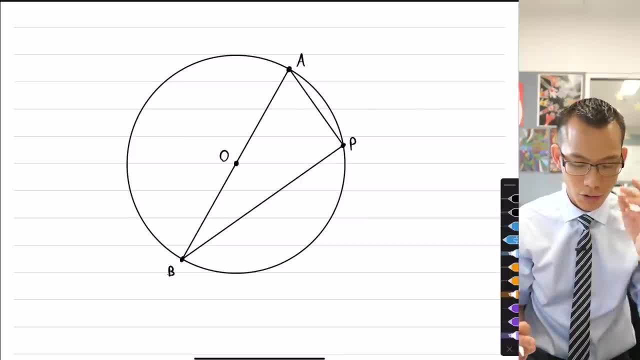 Well, what I'm going to do is I'm just going to put in a small construction and then do some calculation with the angles, some not even calculation, really a bit of manipulation of the angles, and you'll see why. it must be true that A, P, B is right angled. 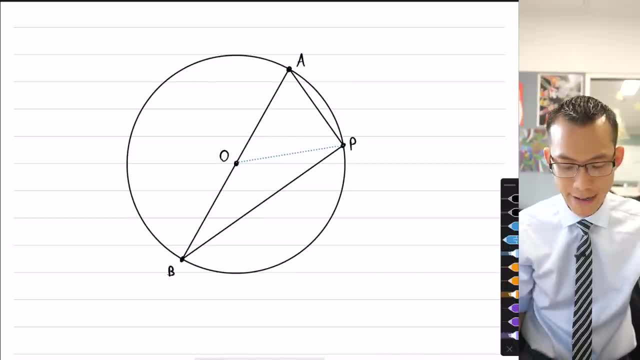 Here's what I'm going to do. I'm going to start by adding in this radius here, OP. The radius OP is valuable because it's not the only radius that I have in this diagram, right, Because A, B is a diameter. 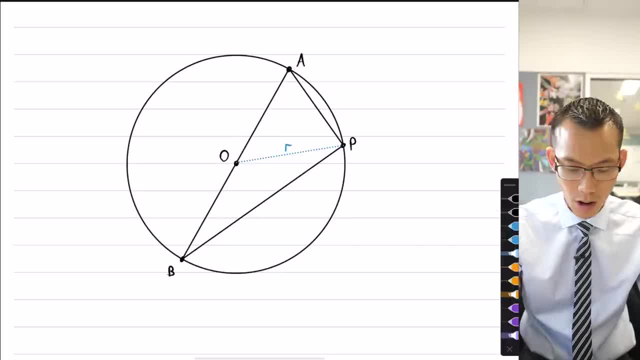 That means that OA that's also a radius, because it's from the center to the circumference, and so is OB. So what I have here is not just the big triangle ABP. I also have two smaller triangles that are both isosceles because they both have radii making up two of their sides. 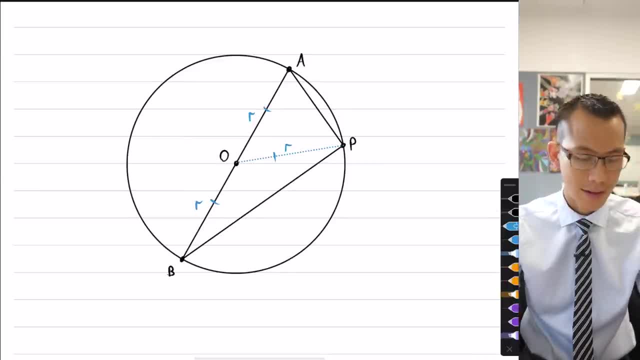 So here's an isosceles triangle here, and then there's another isosceles triangle here. Now, what this gives me is a bunch of angles that I know are going to be equal, because equal sides are opposite equal angles, or in fact the other way around, because the 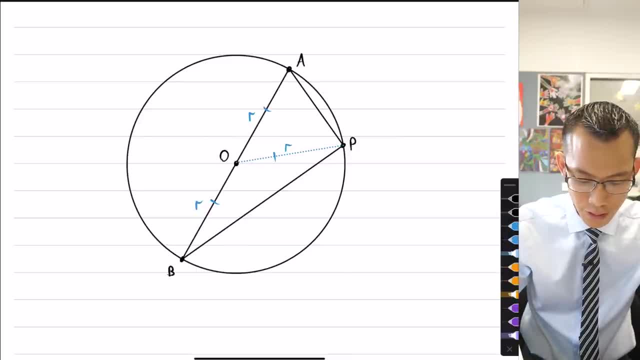 thing that I know is the equal sides. So, for instance, if I focus in on triangle AOP, you can see that this radius is opposite this side, this radius is opposite that side. So I've got a couple of angles that are equal there. 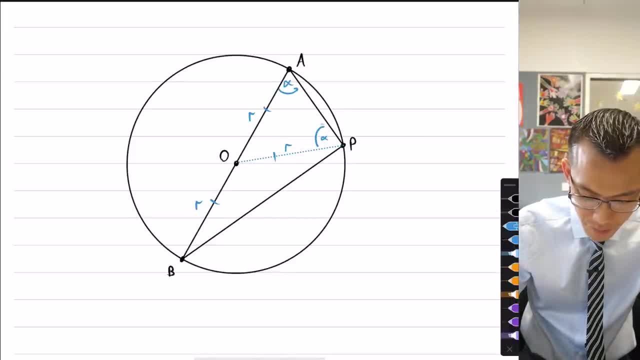 Let's just give them a name. Let's call them both alpha, like so, and then I can make the same argument. let's switch over colors with the other isosceles triangle. right, It's going to be. you might call them the base angles of the triangle. 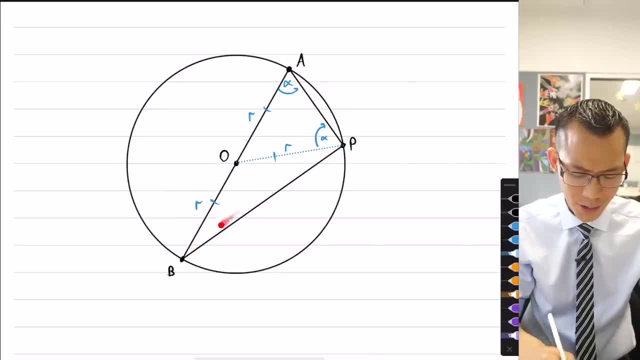 Here and here. Base angles is sort of helpful but also sort of unhelpful. You can see these two angles here don't look anywhere near like the base, which tends to be the bottom of something, because the triangle, of course, can be oriented in any direction. 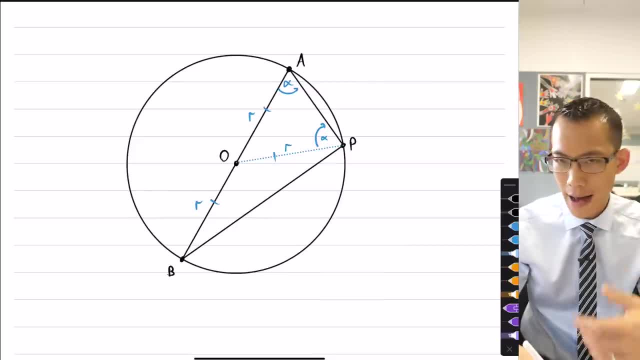 that you'd like. But, by the same token, if I use a different label because they're obviously not the same size, or they're not in this case anyway, I'll call this angle beta and this angle beta as well. Okay, Now I'm only a couple of short steps away. 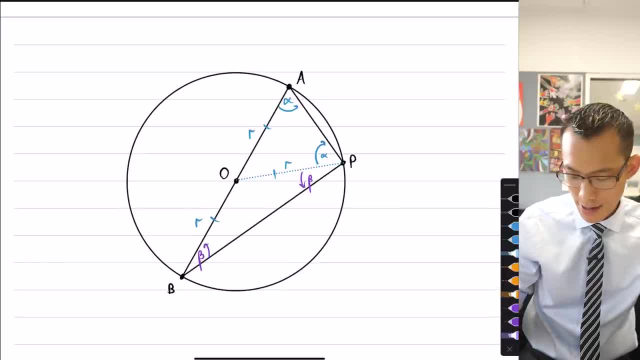 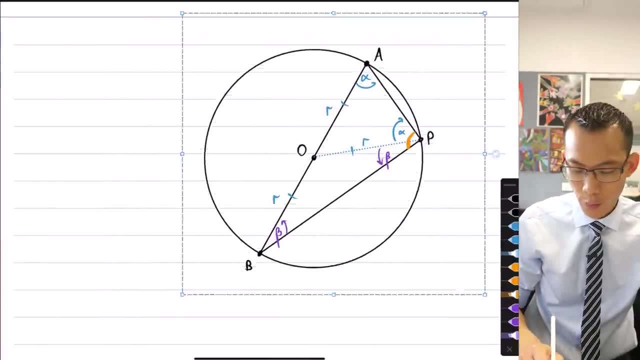 From proving what I wanted, which is that APB. let's mark it in here. This angle here is the one that I'm interested in. I can show that it's equal to 90 degrees in a fairly straightforward way. Maybe you can see the logic before I get there.